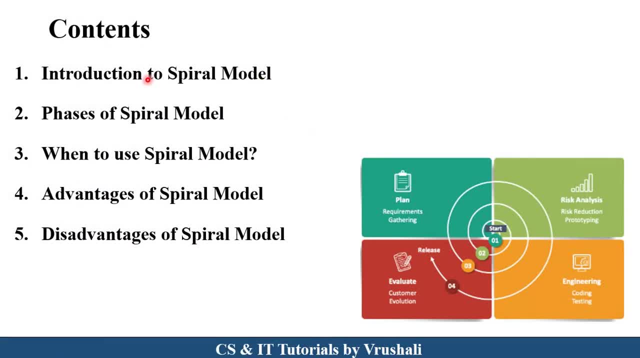 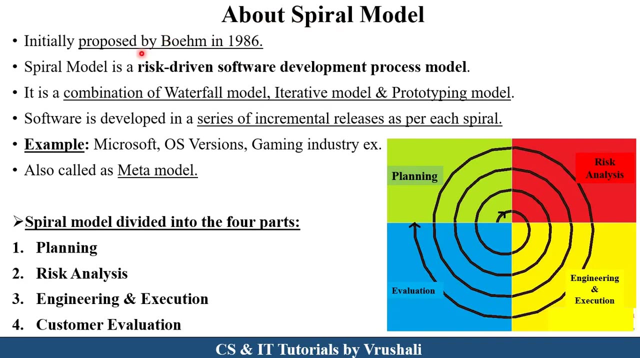 In today's session we will discuss about introduction phases, when to use spiral model and their advantages and disadvantages. Let's see all these points one by one Now. the first point is: what exactly spiral model? Spiral model initially developed by the scientist Bohem in 1986.. Spiral model, which is also called as meta model and spiral model, generally used in large project and the project which have 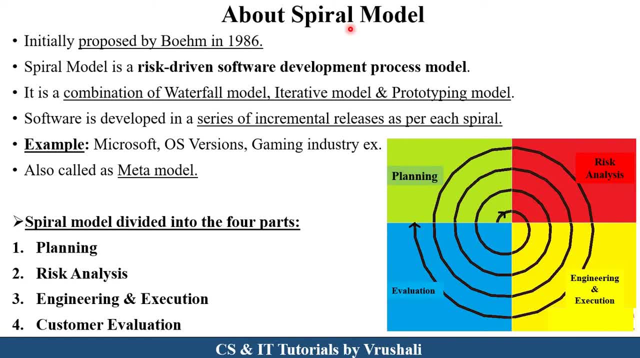 lots of risk and the problem. This is a main area where spiral model have used. That's why this spiral model is also called as risk driven software development process model. Spiral model is a combination of waterfall, iterative and prototyping model. We already discussed these three model in detail in previous sessions. From waterfall model, it take a step by step development approach. From iterative model: it take 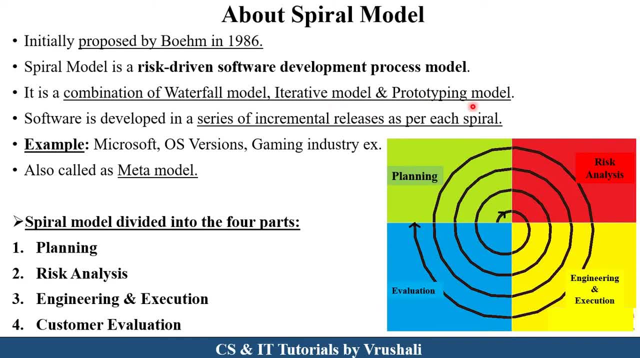 a customer feedback taken approach and from prototyping model it take first developed prototype and then actual development. have started this kind of approach. Next, spiral model generally used in different gaming industry for online gaming. It required lots of customer interaction and lots of risk. is there Next in Microsoft and operating system versions, for example Windows seven, Windows eight and after that windows 1011.. So they use 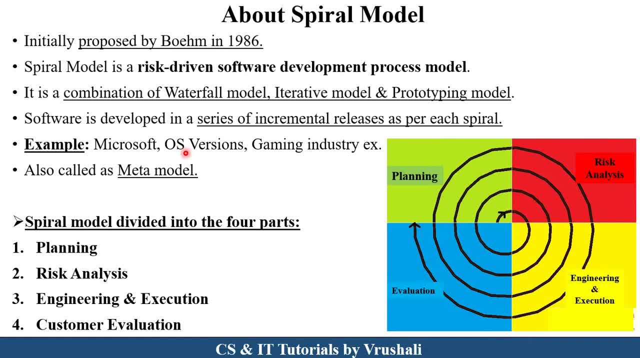 is an incremental approach. they solve disadvantages and risk in previous approach from the next versions right. so in this particular field spiral model have used. see here in this particular diagram spiral model have divided into the four parts: first, planning, second, risk analysis, third, engineering and execution and fourth one, evaluation. let discuss in detail now. see. 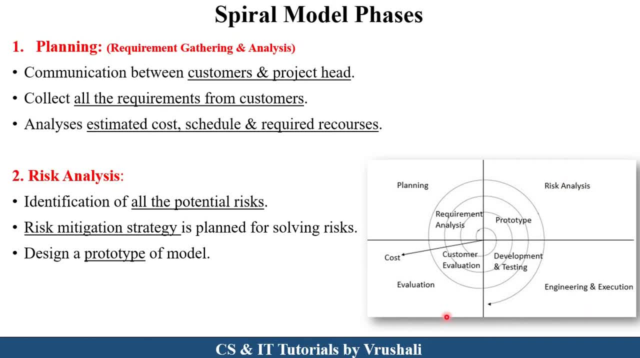 here. this is a actual structure diagram of spiral model. here this particular line indicate a spiral or iterations and it start with this inner point. this is a starting point and this starting point indicate the first phase, that is, planning phase. in planning phase there is a communication between customers and the project head. project head collect all the 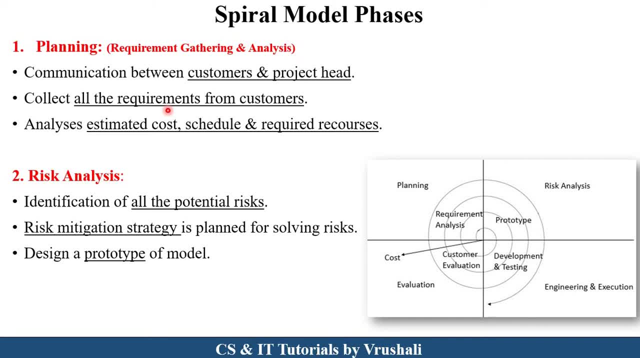 requirements from the customer, what is a need of customer and what exactly customer want. after that, system analysis analyze all these requirements and they decide estimated cost schedule and required resources of the project. now, after collecting all these requirements in the planning phase, it move to next, that is, risk analysis phase. this is the second phase, see spiral model generally. 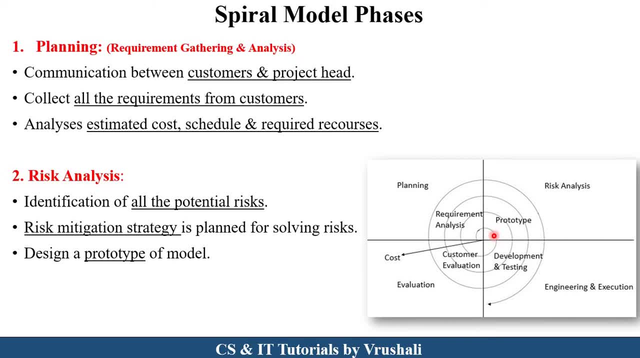 used in large project like ISTRO, NASA. so in that particular phase lots of risk problems and security related issues is there right? that's why risk analysis is the most important phase in spiral model here. the first thing is they identify all the potential risk, the risk related to the technical risk, software and hardware related. 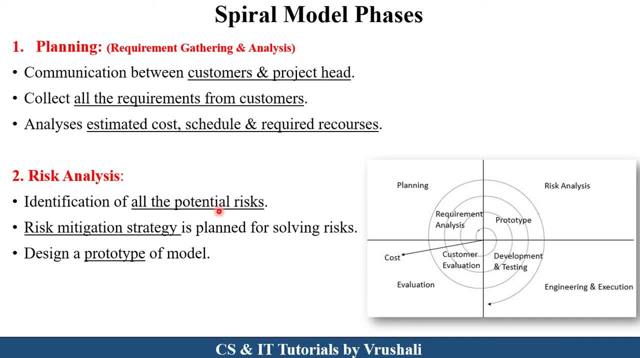 risk or there is a risk in problem statement, in data. so they collect all these types of risk. next they find out the solution for solving this kind of risk or the problem. so this solution is planned in risk mitigation strategy strategy documentation. after that they develop a prototype. so prototype also used for solving. 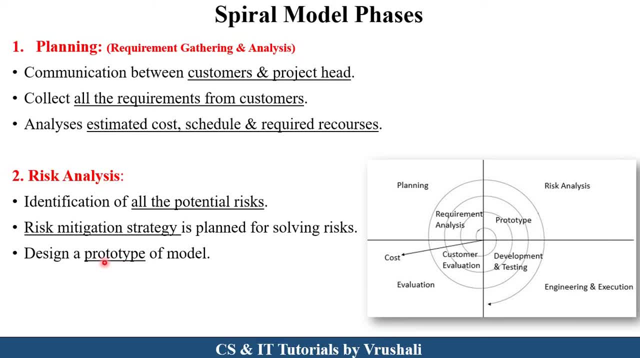 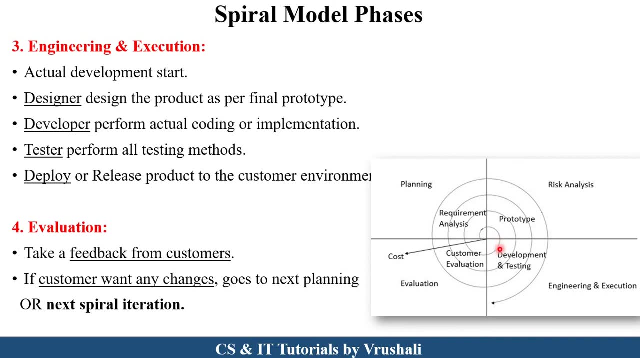 the risk before starting the actual development. first they develop the prototype. prototype is just a replica of your actual software development. so here they develop a prototype. next. now, after developing a prototype, it moved to next phase, that is, engineering and execution. so here actual development have started. first, designer design the product as per the final 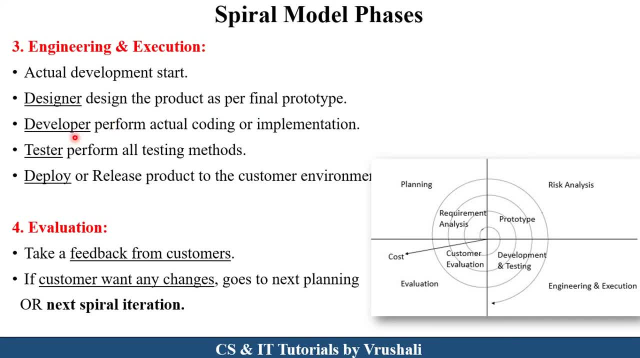 prototype or the requirement. developer perform actual coding by using different programming languages. tester perform testing by using different testing methods. they check whether the project is related to the customer requirements or not. and, last one, after design, coding and testing, they deploy the product to the customer environment. so this is a third. 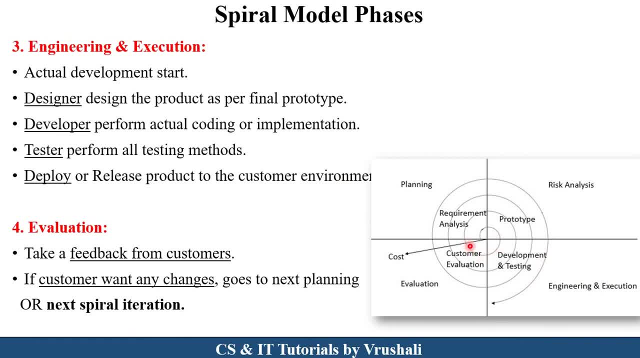 part. now, after deploy, it move to next one. that is customer evaluation. so in this fourth part they take a feedback from customer and if customer want any changes it move to next. spiral iteration means it moves to next one. that is again planning, again risk analysis, again engineering and execution, and 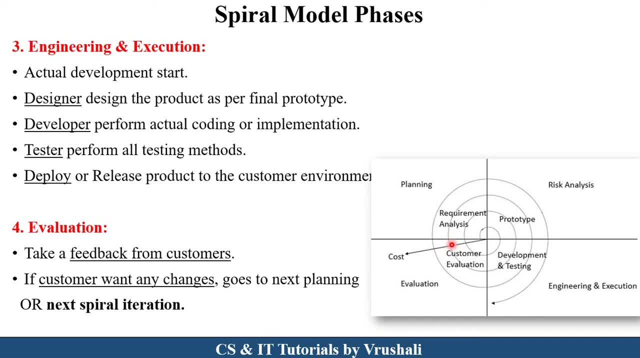 again they take a evaluation means second spiral iteration is there again the check. if there are customer want any suggestions or customer have any needs, so they they again move to planning, risk analysis, engineering and execution. and evaluation in this way means if customer want any changes, it move to next spiral. 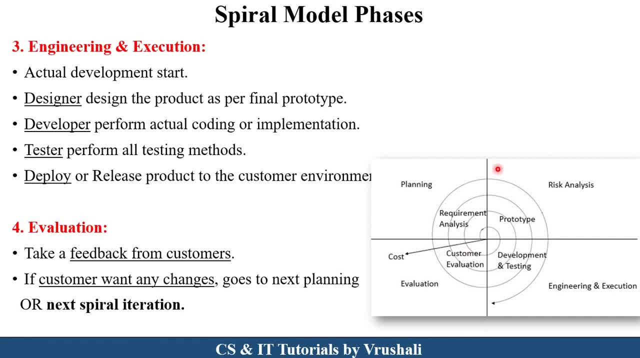 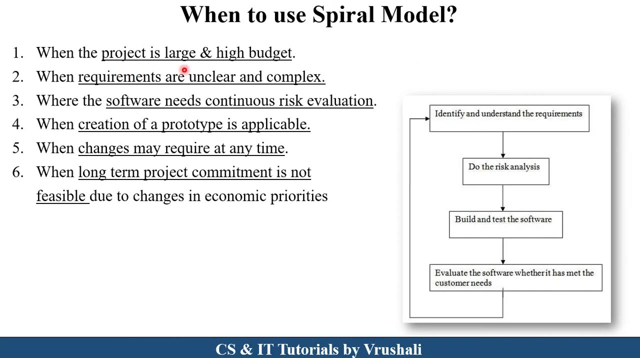 iteration. so the spiral iteration increases means cost of the project increases. and spiral iteration is just one. iteration is there means after one iteration customer doesn't want any changes. customer are satisfied. miss their project. cost is less clear. So this is called a spiral model. Now when to use spiral model? the first, when the project is large. 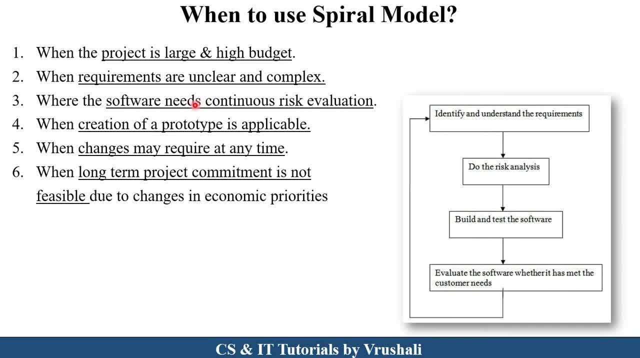 and hybrid project is there? second, here customer requirements are unclear and complex customer requirements. That's why customer requirements are continuously changing, is there? the important thing is here risk evaluation is there? suppose the particular project having lots of risk, So at that time spiral model have used. here they create a prototype. 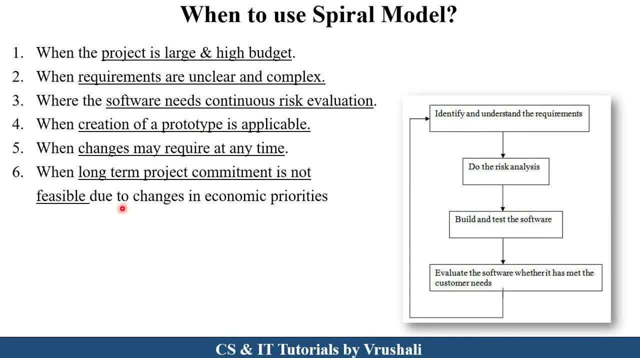 for solving the risk problem. and also there is a no deadline of the project, because if customer requirements are continuously changing, so there is a no deadline. there is a spiral goes to in infinite loop, clear. So in this way, spiral model, have used now the advantages of 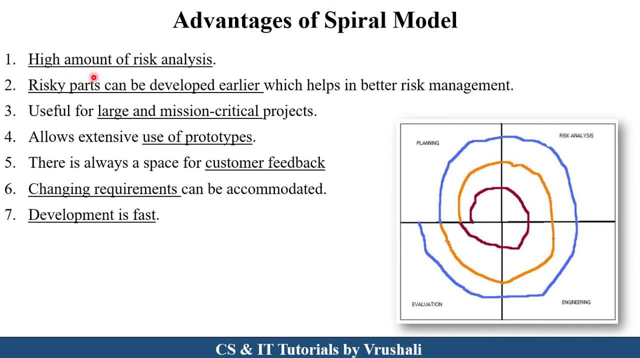 spiral model. The First important advantages is the identify risk and solve the particular risk in particular project. So this risk parts are first develop and then actual development have started. This is the most important advantage. spiral model generally used in large and mission-critical projects. here, after the complete 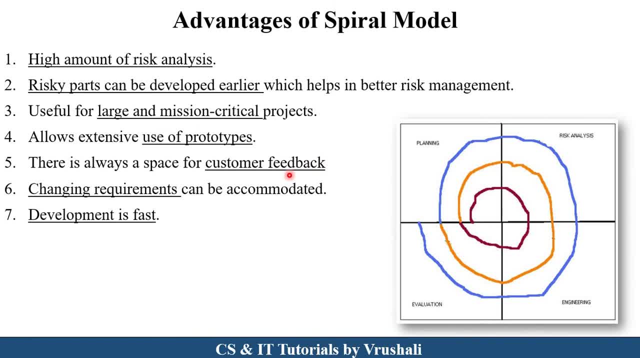 development. customer feedback have taken, so customer interaction is also most important. advantage and customer requirements are continuously changing. not a fixed requirement Is there and they also create a prototype for creating the prototype. it solve all the errors in prototype clear. So these are the advantages.